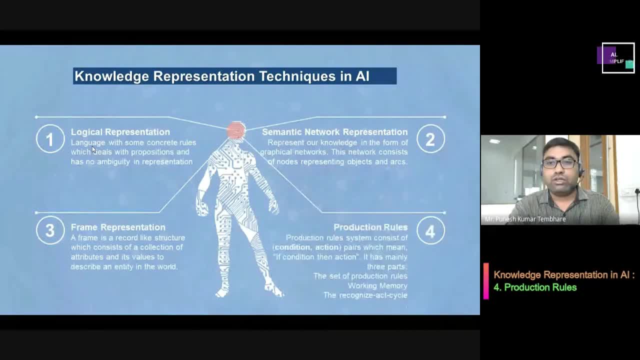 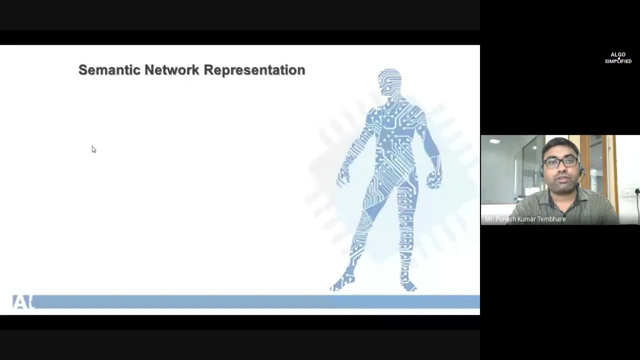 And fourth, knowledge representation technique is a production rules. We have already studied this technique. In this way, we have total 4 techniques to represent the knowledge in Artificial Intelligence And in today's class we have to go for knowledge representation by using 7 Tech Networks. 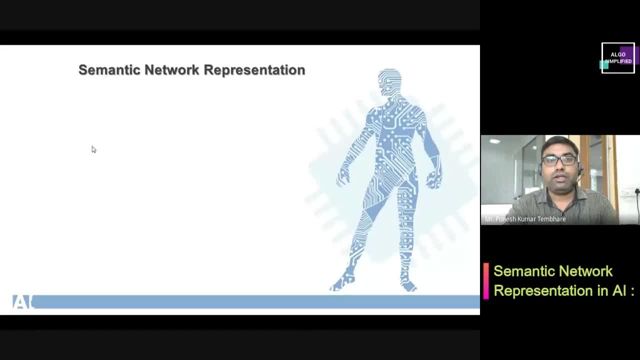 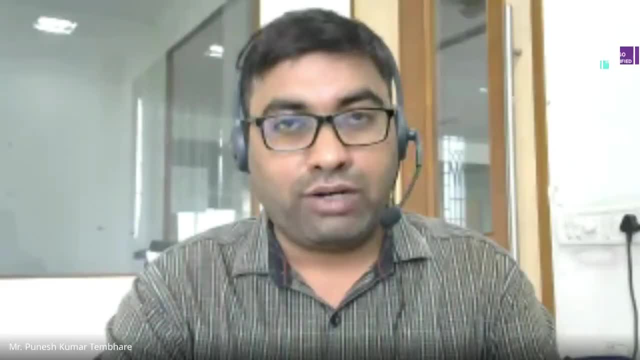 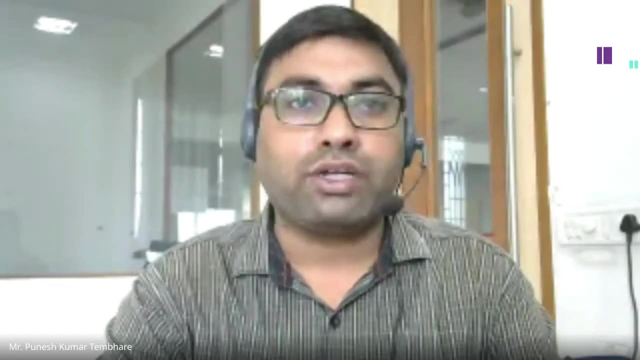 The main idea behind 7 Tech Networks is that the meaning of a concept comes from the way in which it is connected to the other concepts. So, particularly for every concept, we make 7 Tech Networks And according to the way this concept is related to another concept, our network also grows. 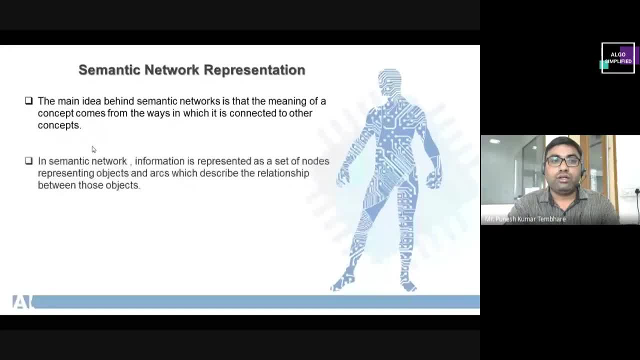 In 7 Tech Networks information is represented as a set of nodes representing the objects and arcs which describe the relationship between those objects. So 7 Tech representation is a graphical representation technique. We generally represent the objects in the form of nodes, Whereas if there is a relationship between the objects, then that relationship will be. 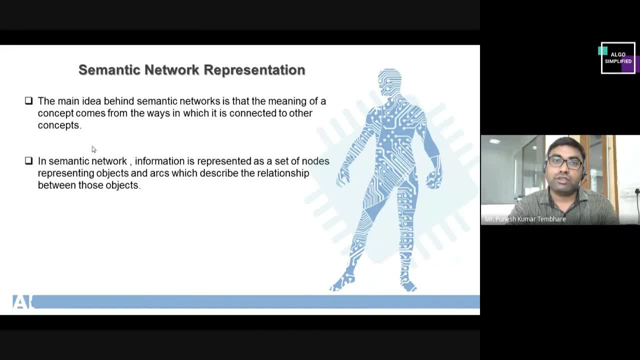 represented with the help of interconnected links in the form of labeled arcs. This representation consists of mainly two types of relation, So particularly easier relation and kind of relation. We represent the relation of these two types in 7 Tech Network representation. So first of all let's understand what is Intersection Search. 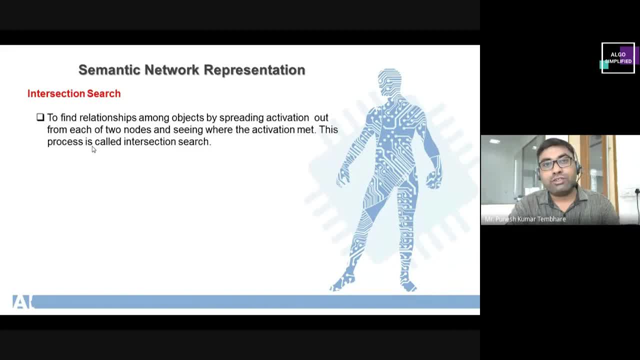 If we have two objects and if the relationship between those two objects is HH and if we want to check, then what will we do? We will simply choose both the objects and we will spread the activation function from both the objects. After spreading both the activation functions, we will check where each other is getting the activation function. 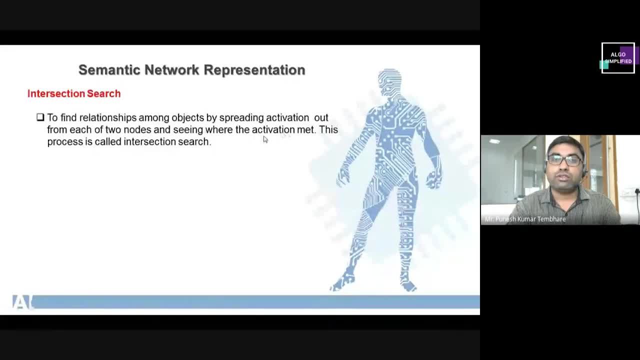 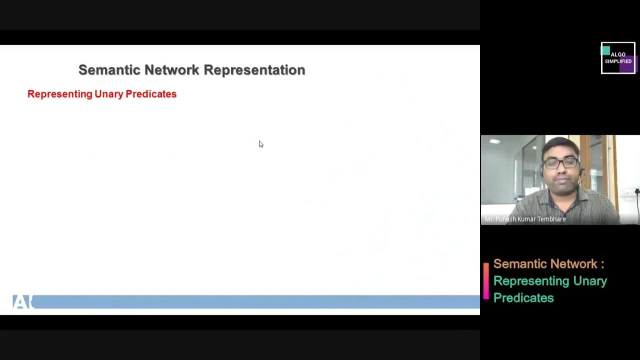 If we are getting the activation function, then it will give us the intersection search. In this way we will get the relationship among two objects. Now you will understand how we represent unary predicates by using the 7 Tech Network. So many unary predicates in predicate logic can be thought as binary predicates using some very general purpose predicates. 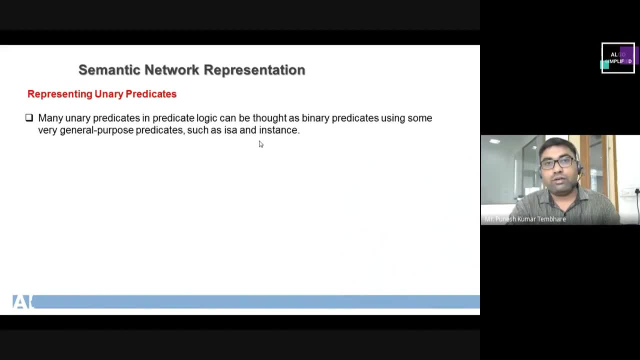 such as each or any instance Generally in the production rule form or in the form of predicate rule. we generally represent knowledge. So we had a unary kind of relationship. So if we want to represent unary relationships in the 7 Tech Network, 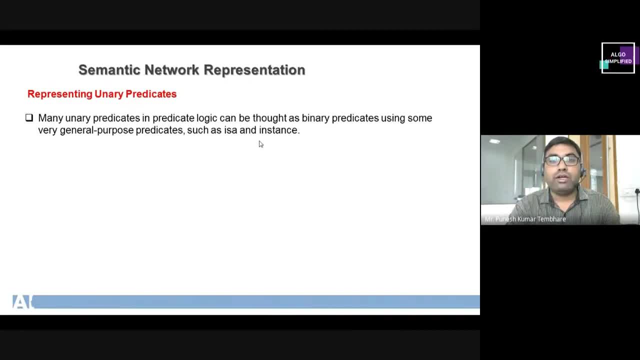 then first of all, we will have to convert these unary representations into binary predicates of each or any instance. We understand this through an example. So here we have an example. For example, the relationship given here is Man-Marcus. So if we talk about the predicate calculus, 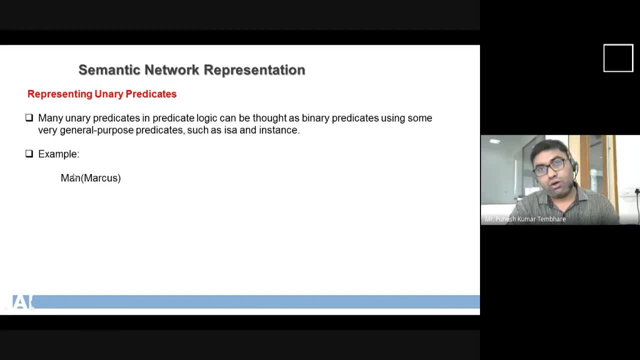 then in the predicate calculus. this is a unary relationship, And now we have to represent this relationship in the form of the 7 Tech Network. So first of all, this relationship has to be taken from the unary form to the binary form. 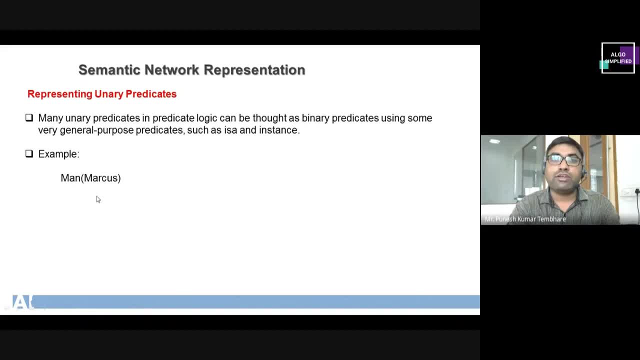 And to take it to the binary form, we have to apply the relationship of each or any instance set here. So how will the relationship between Man and Marcus fall? So, the relationship between Man and Marcus, the relationship which will be there in the binary form, 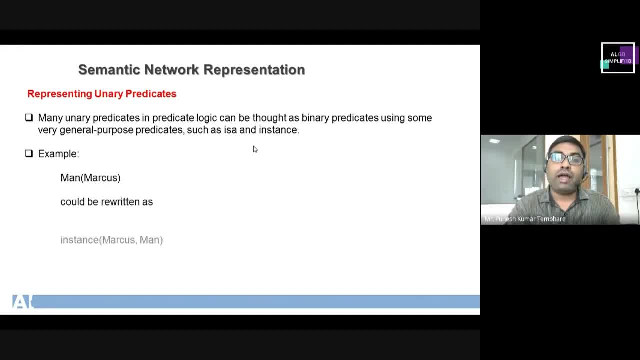 will be your instance type. Why? Because if we have a class named Man, then Marcus can be an instance of Man class, And that's why Man-Marcus, this unary predicate, will be written in this way in the binary relationship. 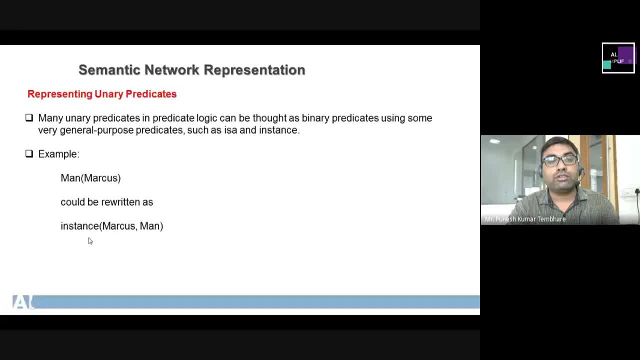 Instance Marcus, Man. And now we have two objects: One is Marcus and the other is Man, And that's why, if we want to represent this in the 7 Tech Network, then first of all we have to make two objects. 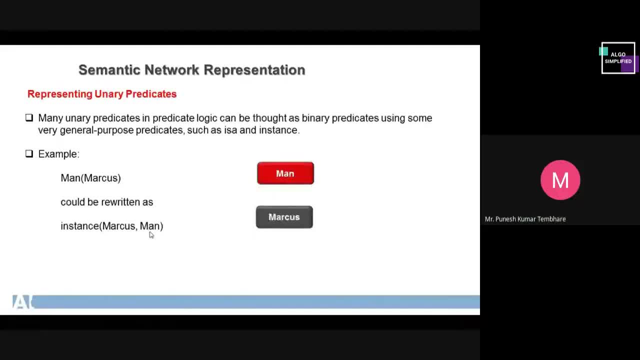 One object will be Man, which we have indicated in the form of one node, And the other object will be Marcus, which we have represented in the form of another node. Now, what is the relationship between the two? Instance relationship? So, what is the instance? 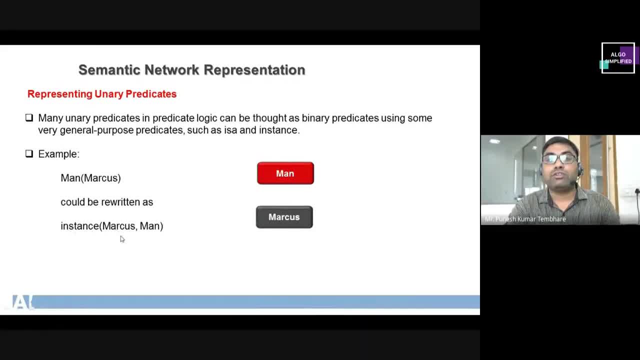 Marcus, And that's why we have to represent this instance- relationship- in a labeled architecture. So if we have a fact of this kind, Man-Marcus, which represents a unary relationship, how will we represent this thing in the 7 Tech Network? 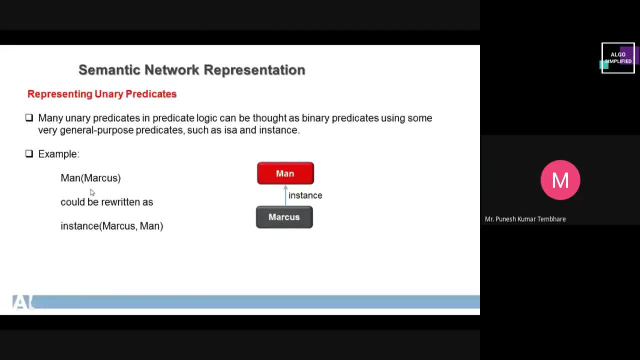 If we want to understand this, then we have demonstrated this thing here. What will we do? First of all, we will convert the unary relationship into binary, And after that we will represent the object and represent the binary relationship in the form of labeled architecture. 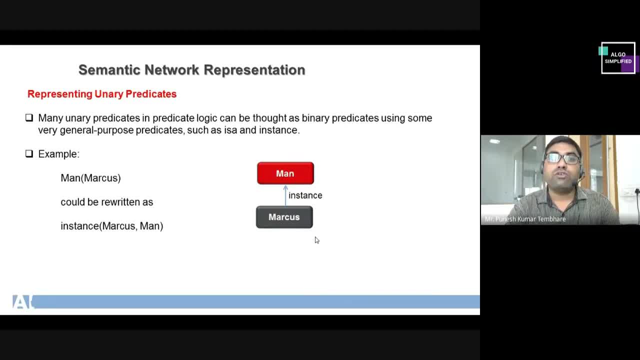 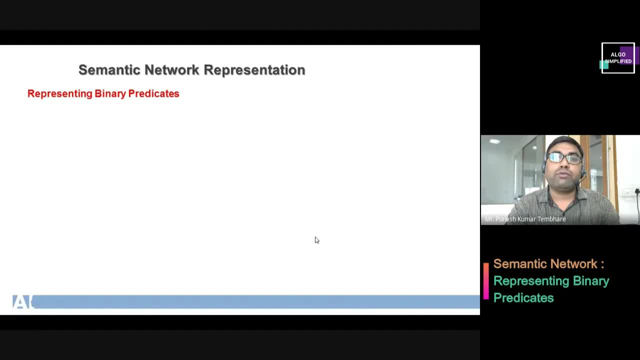 Now we have to understand the concept of how to represent the binary, How to represent the binary predicates. So 7 Tech Networks are natural way to represent the relationships that would appear as ground instances of binary predicates and predicate logic. So particularly, it is very easy to represent binary predicates. 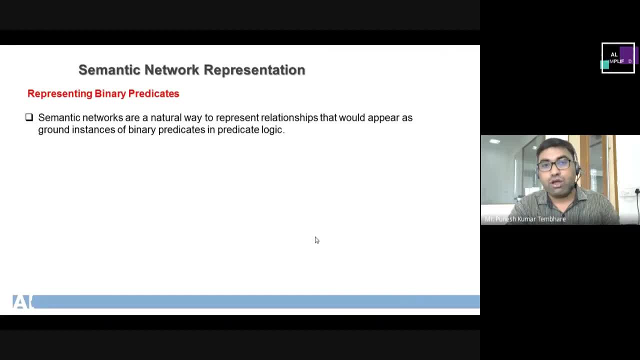 in the 7 Tech Network representation scheme, And we will understand this thing through an example. For example, here we have a binary relationship, Each a person member. So person is a mammal. We will have a fact of this kind. 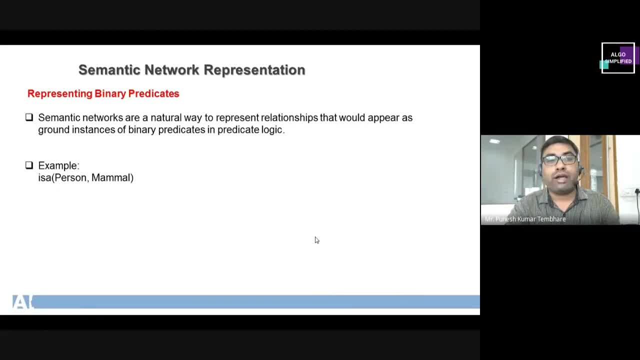 And here the relationship that we have used is a binary relationship, And the object is a person and a mammal. So, simply, we will have to make two objects, which we have represented in the form of a node: a mammal and a person. 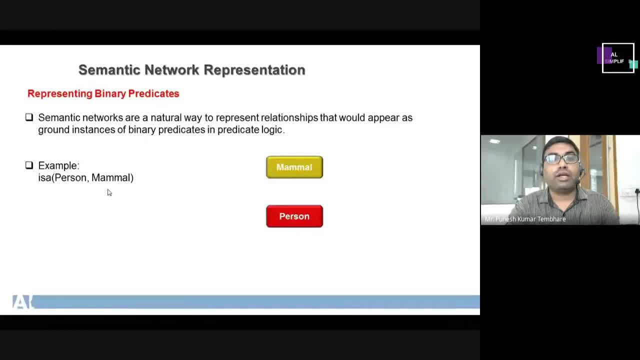 And since it is a binary relationship, we will represent that relationship through a labeled architecture link. Now we have a second binary relationship Instance, such in person. So already we have represented the person as a mammal in the form of a semantic network. 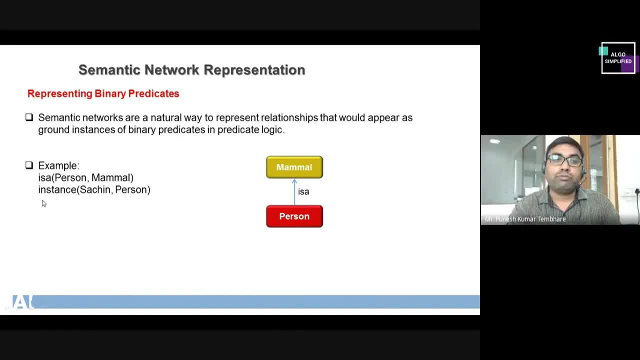 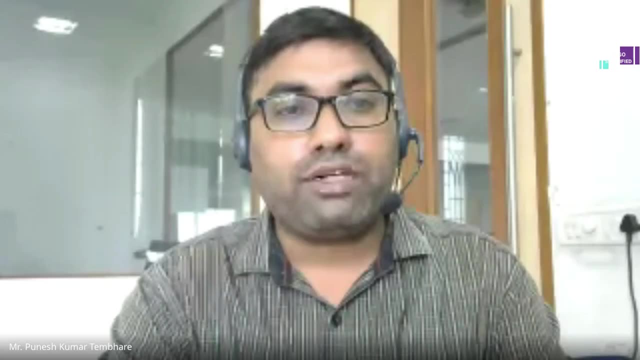 And now our second relationship is such in person, And that's why, if we want to represent this particular relationship, then we will have to extend the previous concept, ie our previous concept. Why? Because we have already talked about the mammal and the person. 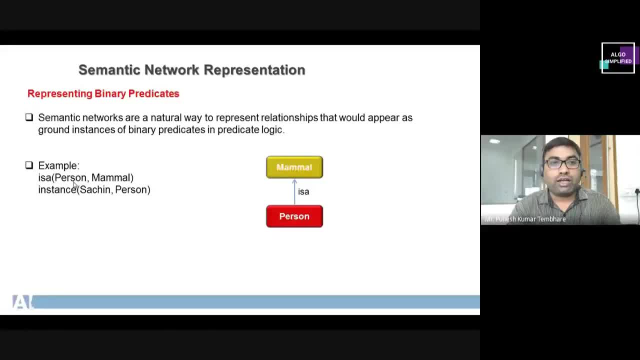 And the person class that we are talking about. a new instance of that person class is coming here, Sachin, And that's why, if we want to add this particular relationship into the existing semantic network, then simply we will have to extend the previous or earlier semantic network here. 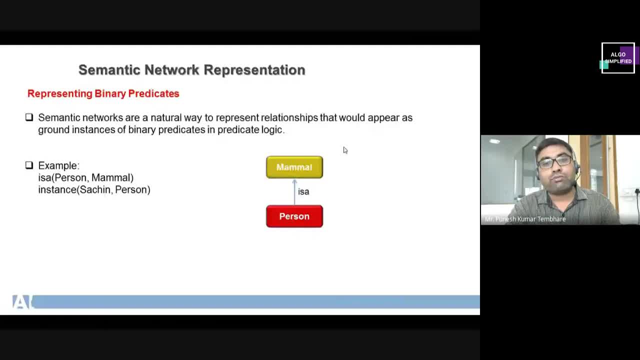 So we can show this relationship in the existing semantic network in this way. So we will have to create a new object named Sachin, And the relationship that Sachin is an instance of person can be shown in this way. Then we have the next relationship. 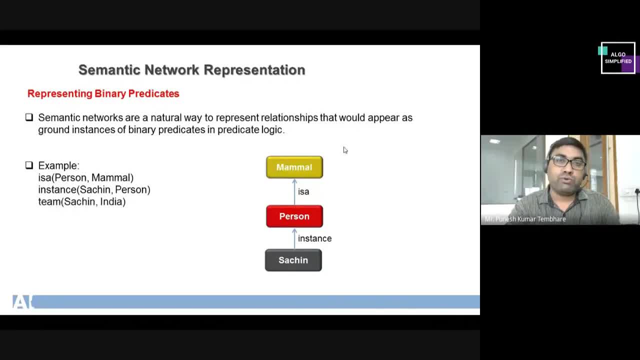 Sachin team is India, So there is a team named India And in that Indian team if Sachin is a player, then if we have a relationship like this, then we will add this relationship to the existing semantic network in this way. 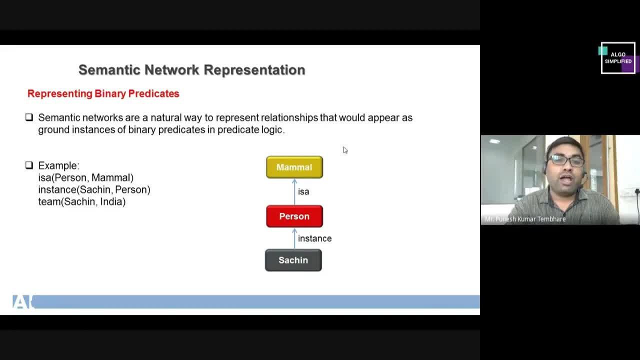 So we have added the object named India again, And Sachin team is India. in this way, We have represented this particular fact in this way. Then we have the next relationship: Uniform: Sachin blue And Sachin's uniform is blue. 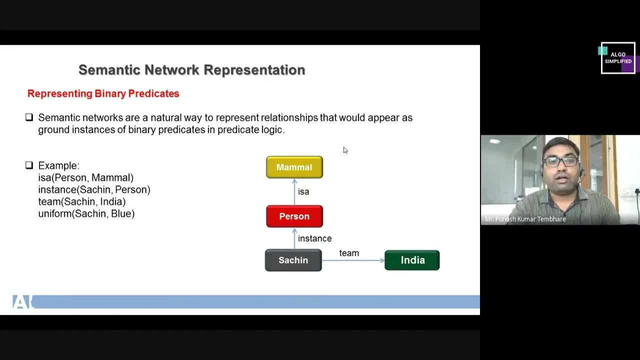 And that's why we will have to create a new object, again blue, And Sachin uniform is blue. We will have to represent this thing in this way, Getting it. So this is about how to represent the binary predicates. Now we have to understand how to represent non-binary predicates. 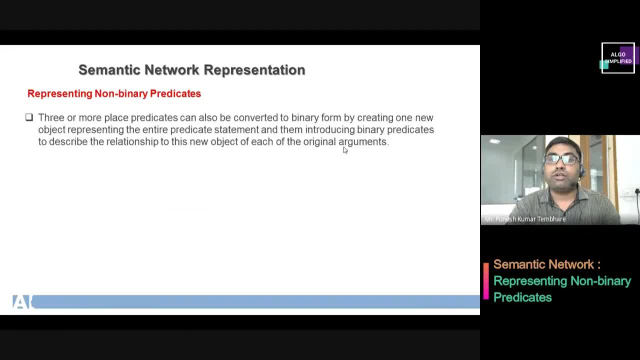 So three or more plus predicates can also be converted to binary form by creating one new object representing the entire predicate statement and then introducing binary predicates to describe the relationship to this new object of each of the original arguments. How did you understand this? Through an example? 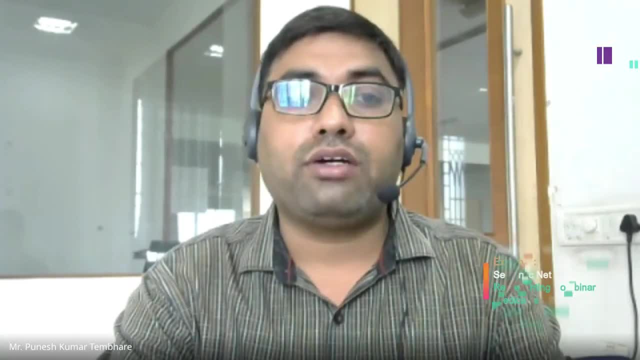 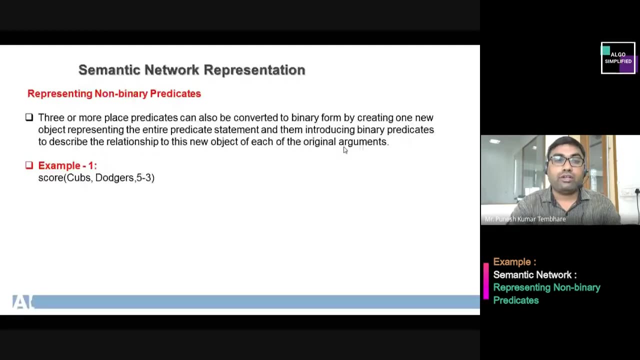 For example, we have given a ternary relationship here. Score Perks, Dodgers 5-3.. So particularly the relationship given here is neither unary nor binary. Now, this is a ternary type of relationship And when we have to represent these types of relationships, 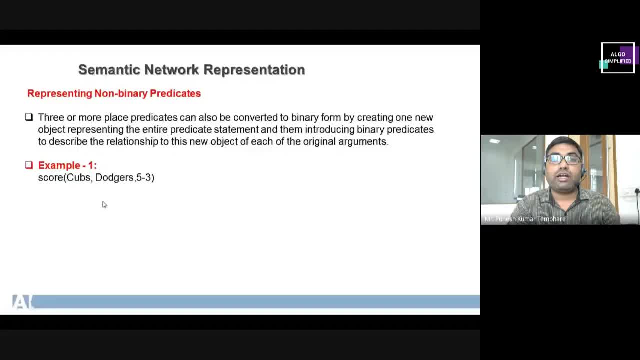 at that time we have to go for the event creation. For example, we have created an event here. G23 is the instance of a game And the relationship is an easy relationship, And then Dodgers. after that, our new object will be 5-3.. 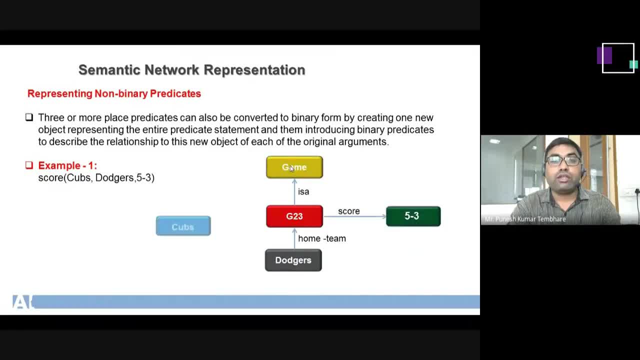 And one more object will be curves. We will have to create all these objects first And after creating, we will have to create the binary relationships between them. So whenever we create non-binary relationships, if we want to represent non-binary predicates, 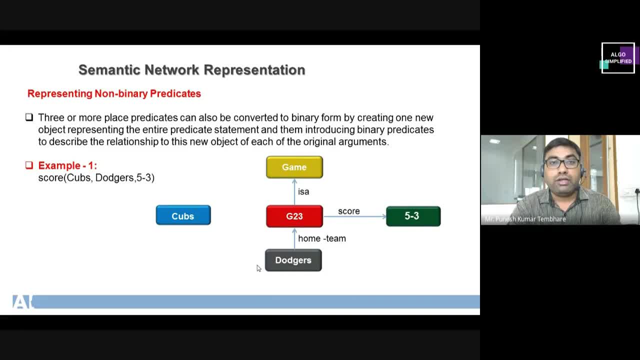 then at that time, to represent non-binary predicates, we will have to add multiple binary relationships to our semantic network. So for example, score curves Dodgers 5-3.. If we have any relationship here, there will be multiple binary relationships here. 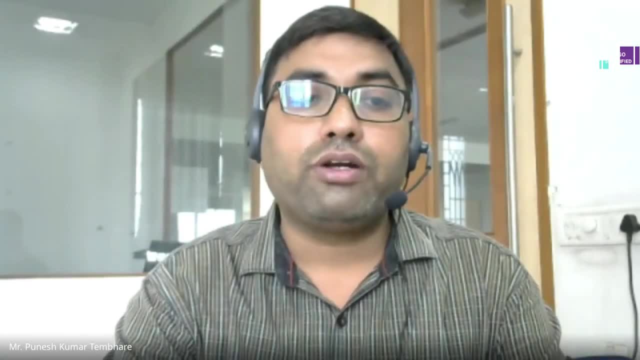 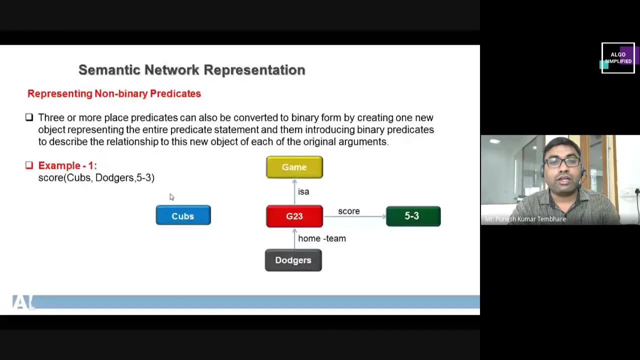 So if we want to represent this particular fact, then to represent this particular fact after creating the event, we will have to create multiple binary relationships here. For example, our score was 5-3.. Dodgers was the home team, Curves was the visiting team. 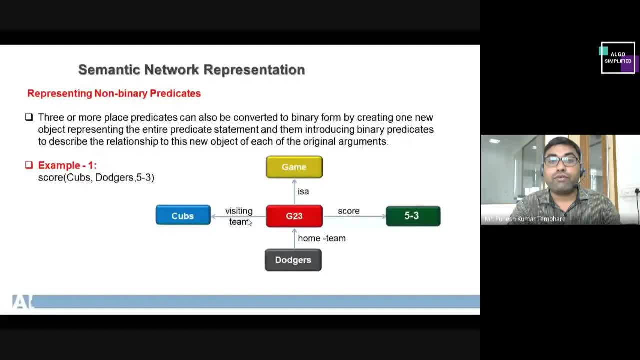 And we are talking about this particular game And the game's particular instance was G23. So in this way, by creating events or instances like this, we have to represent non-binary predicates generally. The same thing Again. we will understand through an example. 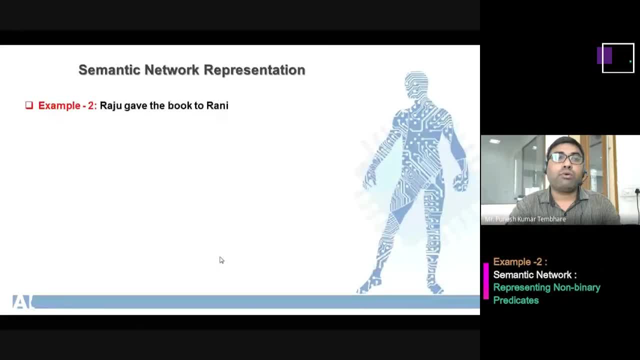 So we have a new example, Example 2. Raju gave the book to Rani. Raju gave the book to Rani. Now look here: One object is Raju, The other is Rani And the other is the book. 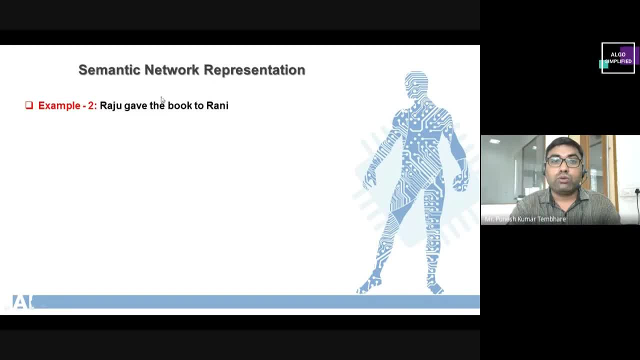 So somewhere here there is a terminal type relationship And if you want to represent this relationship through semantic network, then at that time again you will have to create multiple binary relationships And these multiple binary relationships will have to be added to your semantic network. 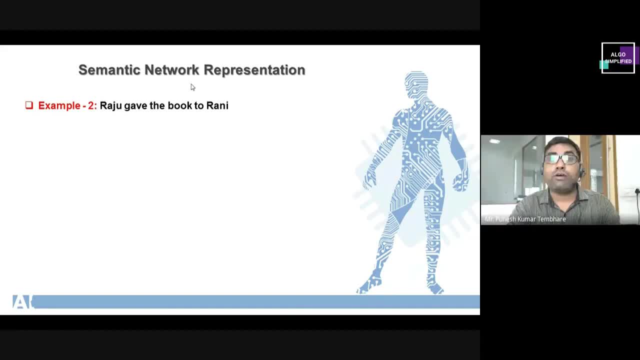 And as the concepts will move ahead of you, accordingly you will have to increase your semantic network Very first. you will have to create an event or instance here, And that's why the first thing is: which objects are our objects? 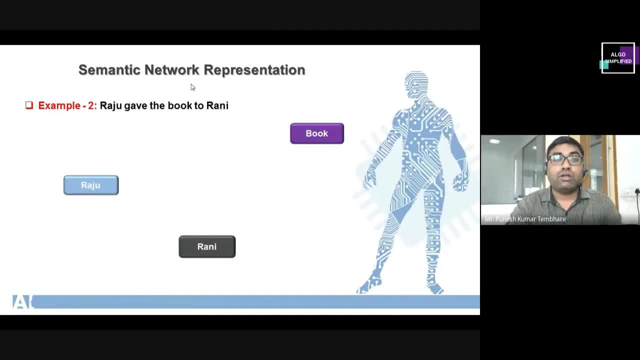 Which objects are these particular facts? If we see, then the objects are Raju, one is the book and one is Rani. So Raju, Rani, book, And there is an event happening between them. And what is that event? 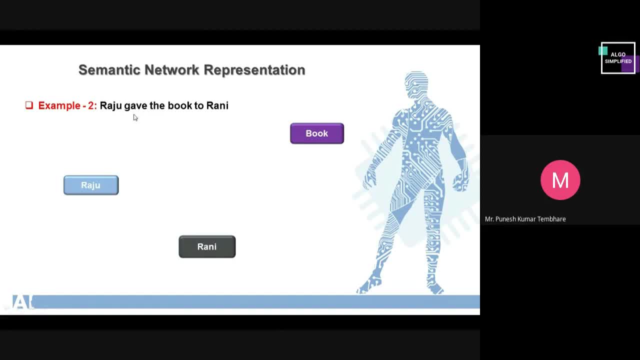 What is that event? It is an action, It is a game, But it is a giving mechanism And we have to create an event of a giving mechanism here. That's why, if you see, then by creating an object we have created an instance of it. 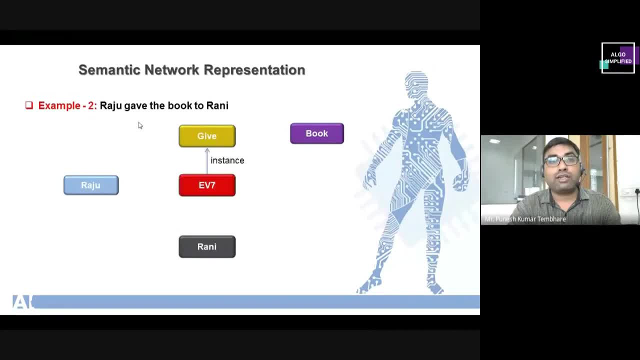 here UV7. And all of our objects are related to this UV7 mechanism And we will add them too. And by adding them, whatever can be our multiple binary relationships, we will create all of them here. So we have created an event here. 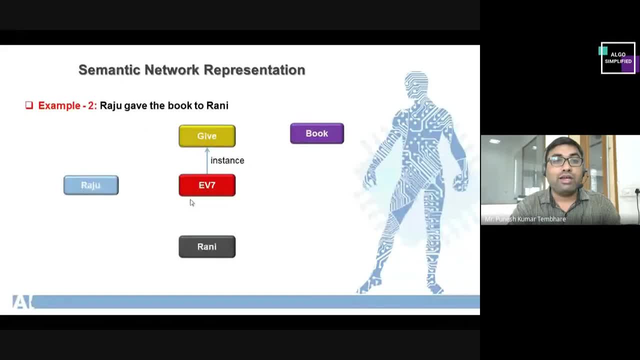 The event UV7, is an instance of giving mechanism. And who is it happening between? It is happening between Raju and Rani. And because of which object? Because of the book object. So the book is also a class of all the books in the world. 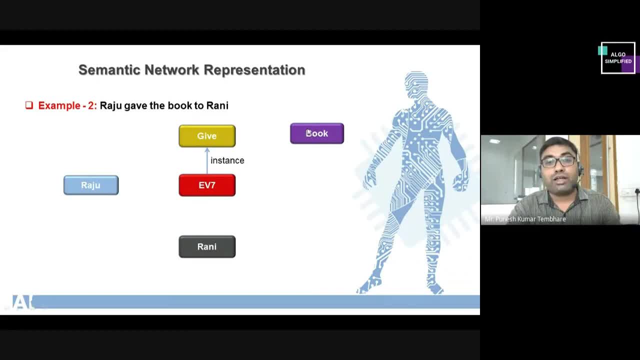 And if we talk about a particular book from that book, then we will have to bring an instance relationship here again. So you can see that we have created an instance called BK23.. The book is indicating here about all the books in the world. 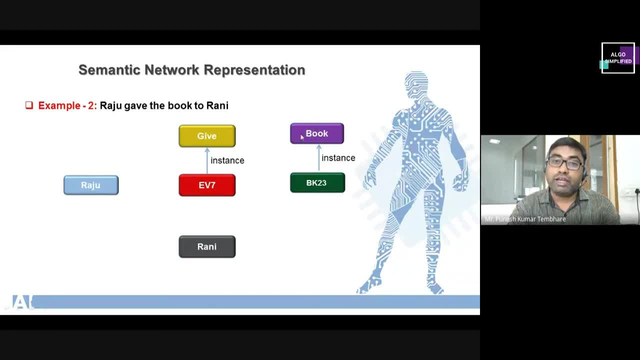 But it is talking about a particular book from all the books, And that book is BK23.. And now this event which is happening is happening between Raju Rani and that book's instance, And that's why, now, what is the book? 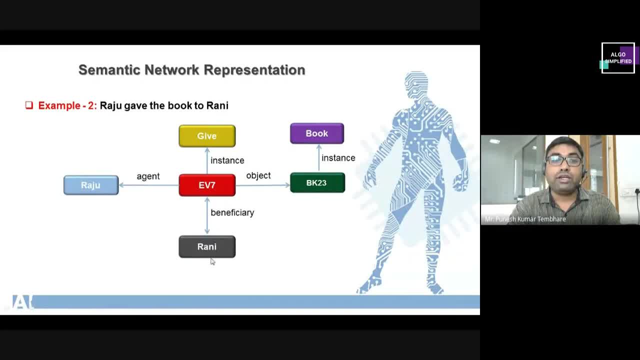 It is an object. Who is Rani? It is a beneficiary. And who is the agent? It is Raju. In this way, Raju gave the book to Rani. This particular fact can be represented through semantic network. So this was about how to represent the non-binary predicates in semantic network. 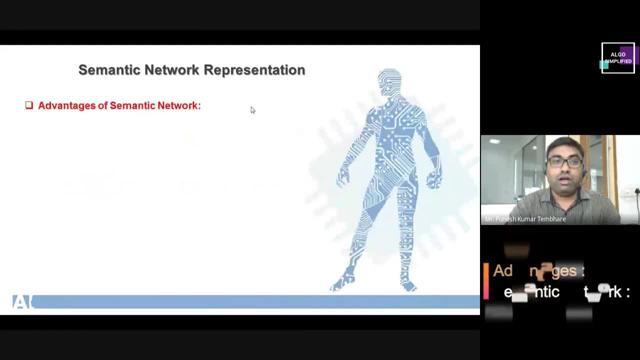 Now we have to understand some of the advantages of semantic network. The first advantage is: semantic network is a natural representation of knowledge. So, particularly according to the concepts that are coming, we are simply representing our data graphically. Semantic networks convey a meaning in a transparent manner. 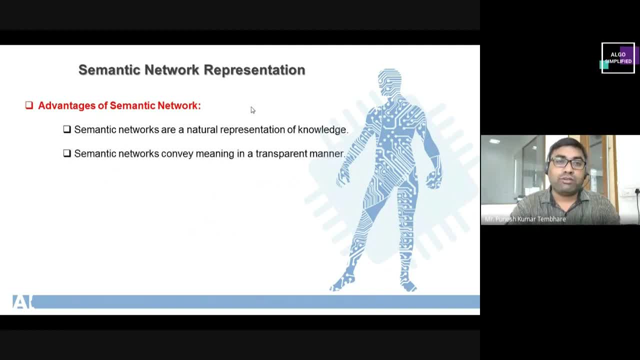 which we just understood. And third, these networks are simple and easily understandable. So if we see the simple mechanism in semantic network, then we are representing the knowledge in a very natural way, in a very transparent manner, And this mechanism is easy to understand. 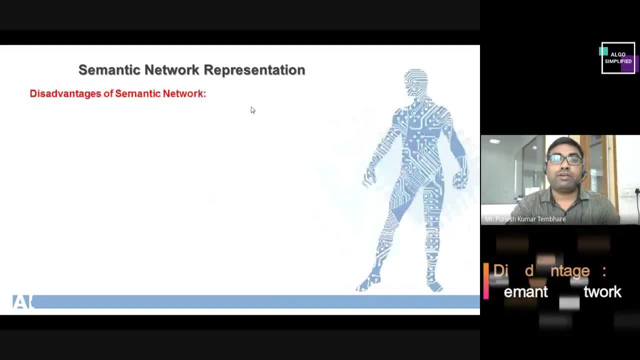 Now we have to understand the disadvantages of semantic network. First disadvantage is semantic network takes more computational time at runtime as we need to traverse the complete network tree to answer some question. So, particularly if we have represented knowledge in the form of semantic network, 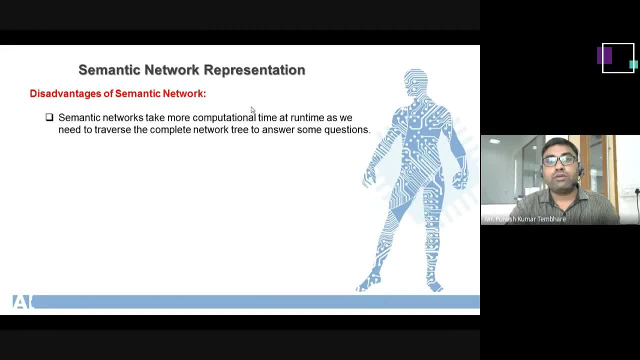 and whenever we perform reasoning. and if we perform reasoning, if we have to search for information, then while searching for information, we have to search for the entire semantic network, And that's why, in most case scenario, it is possible that all the semantic networks 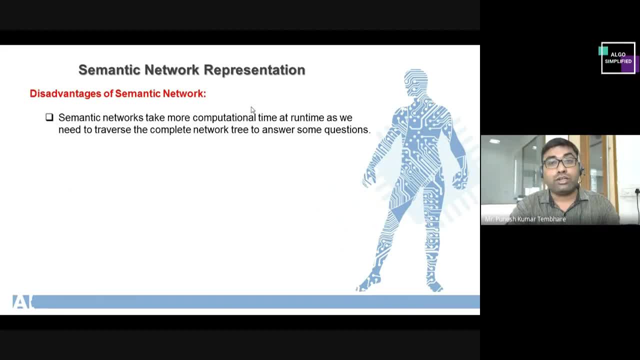 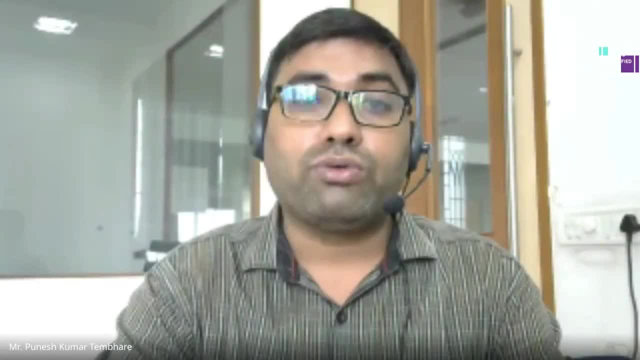 all the semantic networks, we have to search for them. Their searching will be very exhaustive And that's why if we talk about the runtime, computational time, then the computational time will be very long here. So generally, if we talk about human beings, 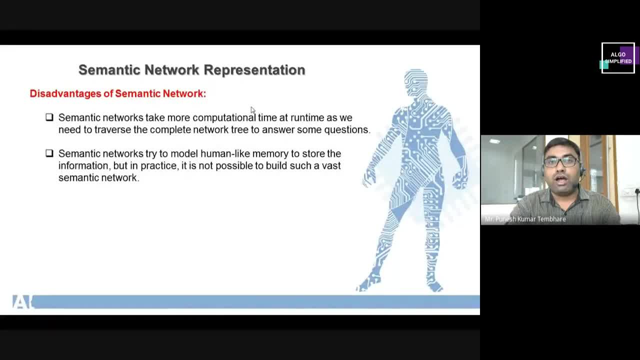 then all the knowledge in our human brain is stored in the form of neural network And in a similar fashion we are talking about creating the same type of network here, But that type of neural network totally it will be very difficult to simulate here. 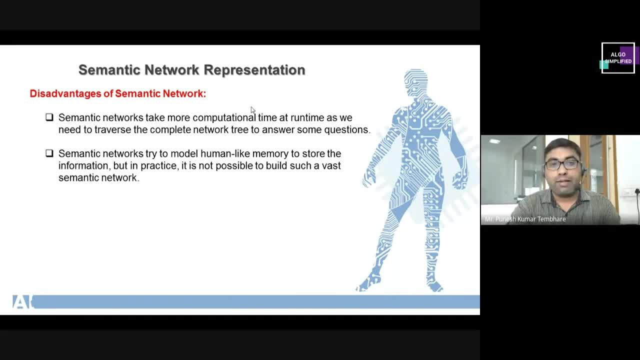 This is what the second disadvantage of semantic network. Then, third, we have: if we use semantic network, then while using semantic network, the quantifiers, like for all quantifier or for some quantifier, it is very difficult to represent such quantifier statements. 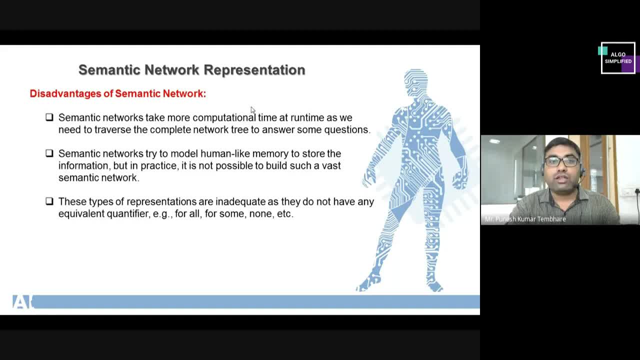 So we can say that semantic network representation is unable to represent the quantifier statement. Fourth, our disadvantage is that semantic networks do not have any standard definition for the links, Generally all the objects which have relationships. how will they give a standard name to these relationships? 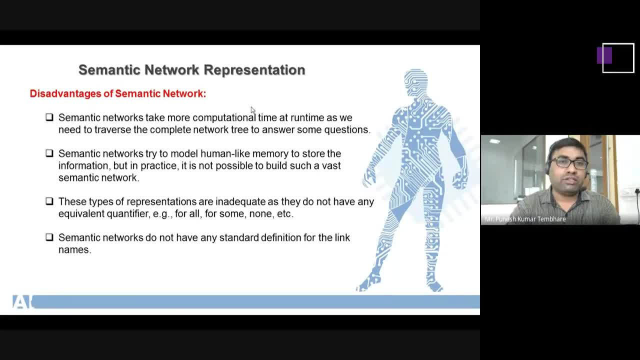 We don't have a fixed mechanism. This is what the next disadvantage of semantic network- And we have last disadvantage, These networks are not intelligent and depend on the creator of the system. Particularly, the cleverness of semantic network depends on who makes it.